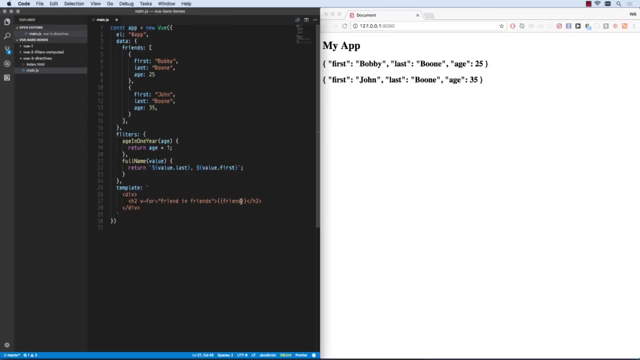 javascript object for each person. Oh great, although that's not really what we need. We want friend name. Actually, there's no such thing as friend name, Friend first, Or in this case we could also do friend full name. So it'll again, we can use the filter on each object. 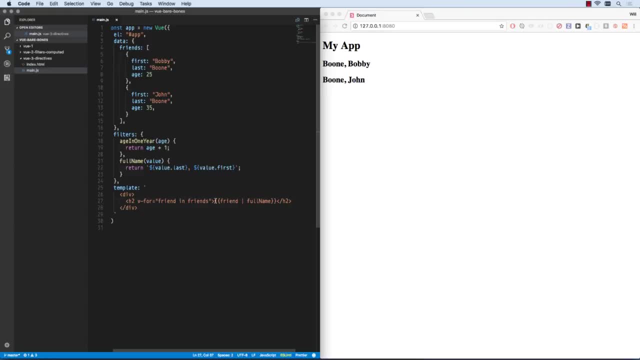 that works just fine here as well. so that's the v4 directive. let's also say: we want to start changing friends names. we want to be able to edit each friends name. so what I'll do here is I'll create their name in an h4 and let's create an. 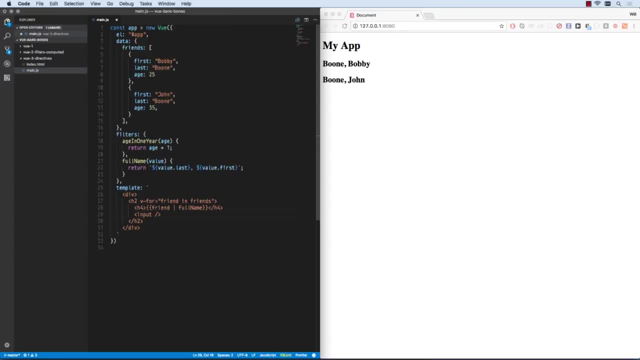 input and let's actually say we want to edit their first name. so the model is going to be the directive for this and we could see friend dots first, and so v model means that it's automatically going to sync to that first name and when I make changes it's two-way data binding. so if I change the Y, then 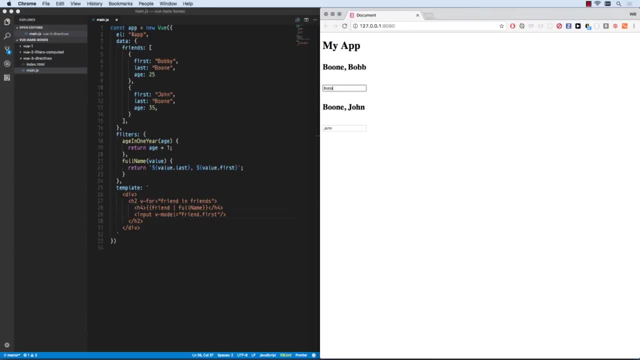 automatically. that got changed. it got changed in my data and that triggered a rear end err on anybody that was listening to that data. so it's reactive to a reactive data binding there. so I can say his name is now Billy and And I can say John's name is Johnny. 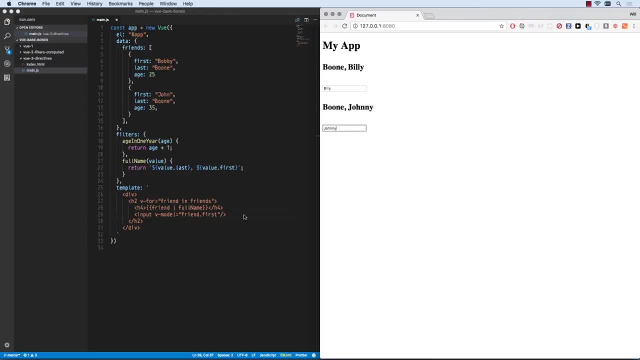 And so that's a really simple way to edit data. That's one of the simple things that makes Vue easy to work with. is that two-way data binding, So let's also make a model for friendlast. You can see now that we can fully edit. 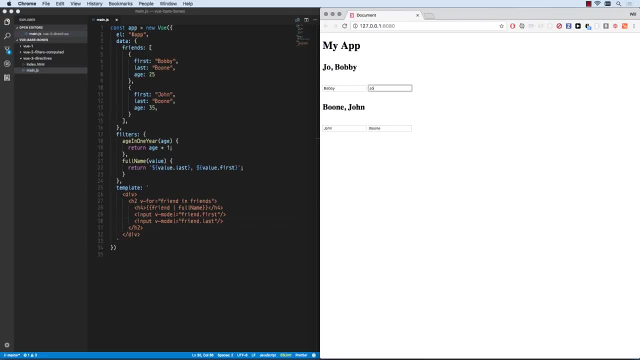 any one of their names. Now let's say we want to work on that person's age, So let's make an H5 for their age. How could we change their age? We can add some buttons to maybe bump it up and down. 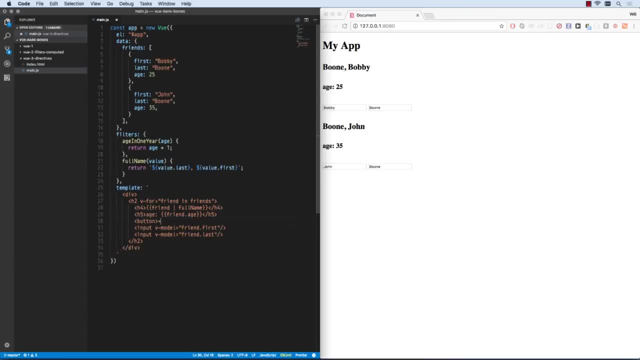 So let's make a button here. Now what we can do is we can use the V on, which will allow us to act on any user event. So the user event we want is a click. So we're going to do colon click. 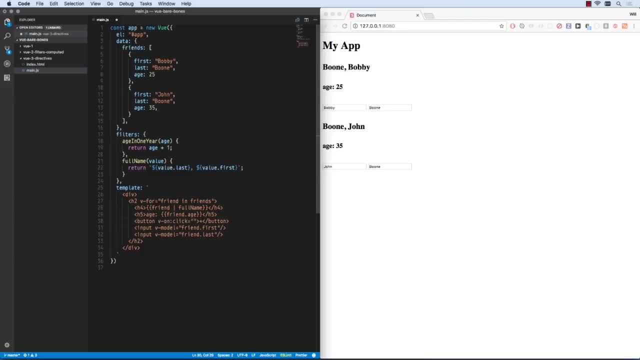 So V on colon click equals, And then We can have it do something. We can say: friend Friendage equals friend age plus 1.. Let's see if this works. Yep, it works. And then I can also make a minus button that 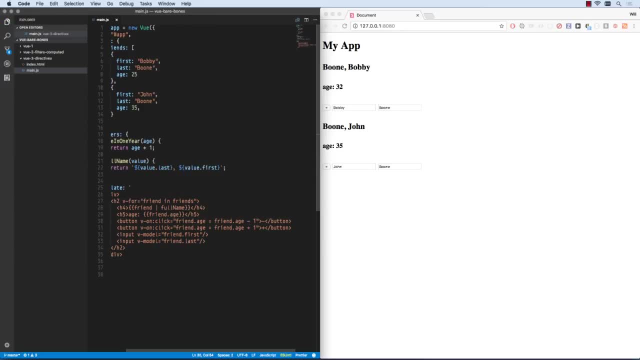 will take their age down. one: We can change their age. change their age back. Change their age back up, change their age back down. Now, while that's a very simple, quick way to do it, the better way of doing this is to move this logic out. 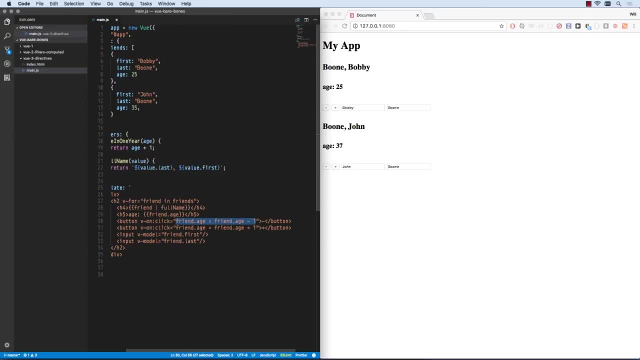 of the template. Logic in a template is, generally speaking, a bad idea. You want to do this as little as possible, So we can add a methods object. now Let's make a methods object And we can say: increment age And this will receive a friend. 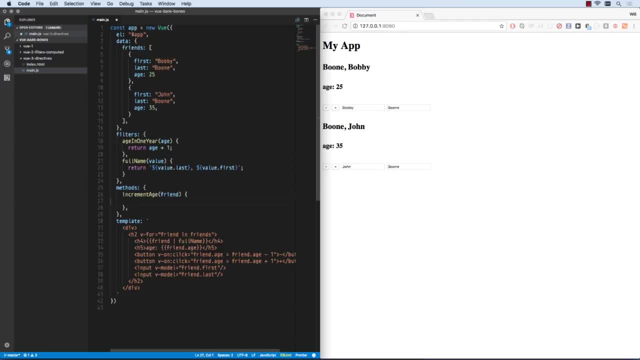 It's very important that we receive a friend, Not just a number, because we can now go: friend age equals friend age plus 1. So what we can do now is, on click we can say, hey, increment friend, And now this will work. 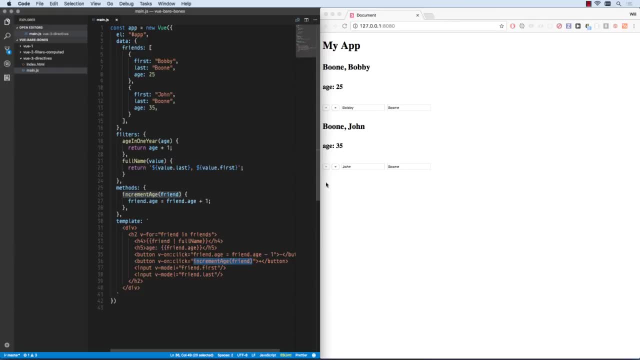 So we are going to increment age. pass it in our friend And then this will automatically bump the age up. You can see up still works and down still works in the hacky way. So let's go ahead. Let's change this to a decrement method now. 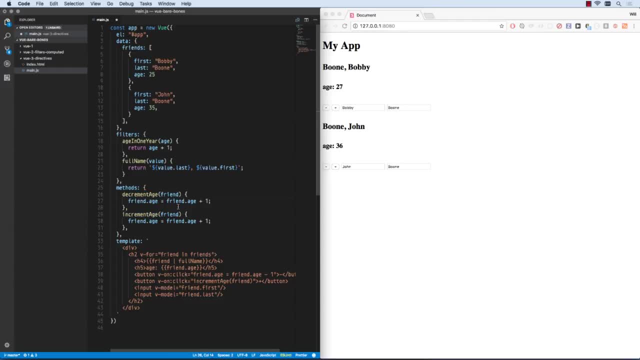 Decrement age, And that will be minus 1.. So then this will be decrement age. So now we're just essentially handing that method off there. We're handling that logic out of the template and into a method. There we are: We're able to change our friend's ages. 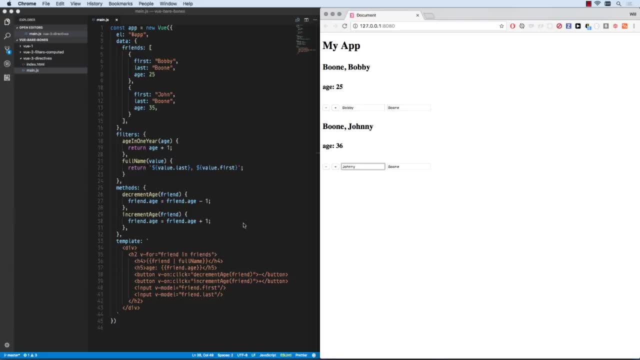 And we're able to change our friend's names. So that's how you work with data, using methods and using directives in Vuejs.